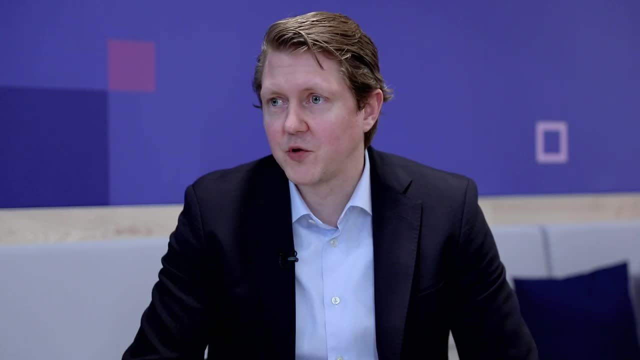 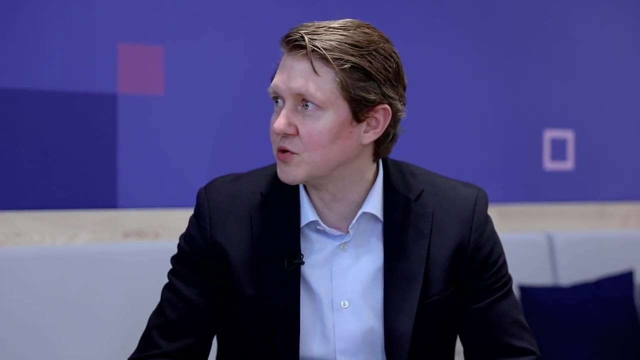 Yes, It's been a very interesting journey. actually, We are, of course, as part of our portfolio, we always have an important software component, But we have realized that on our own proprietary hardware, We have always had a tight connection between the hardware and the software. 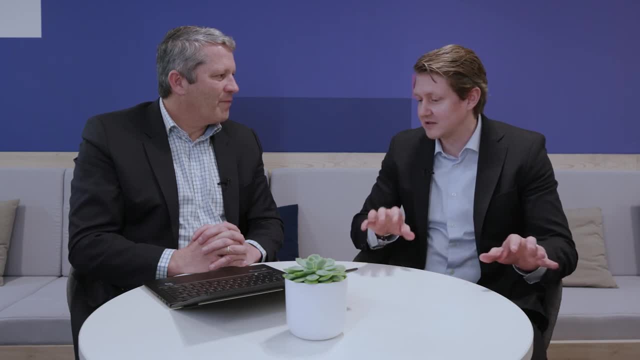 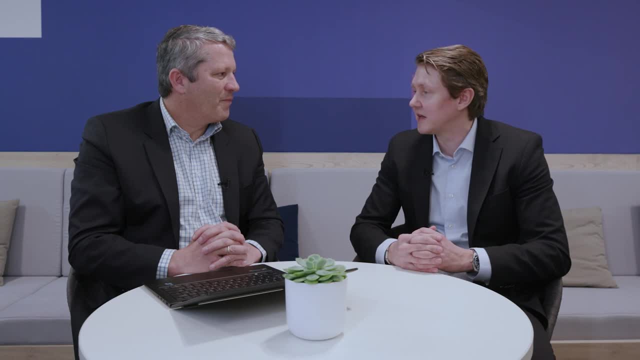 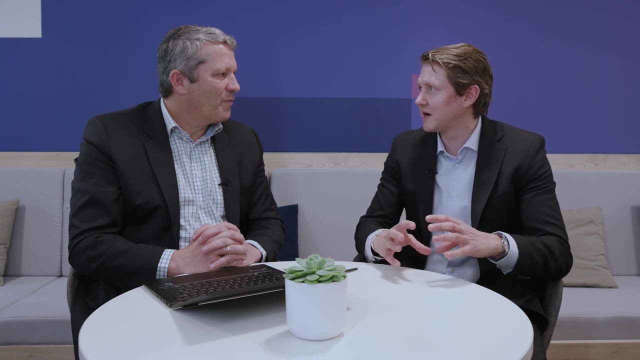 we're working on the software, So we're working on the software, So we're working with hardware vendors- some like CPU and accelerators, such as yourself, to realize the solution. So that means that we are separating our development in terms of cloud run to software business only, and then we 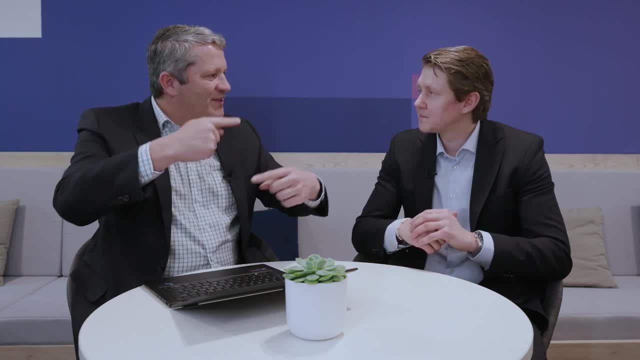 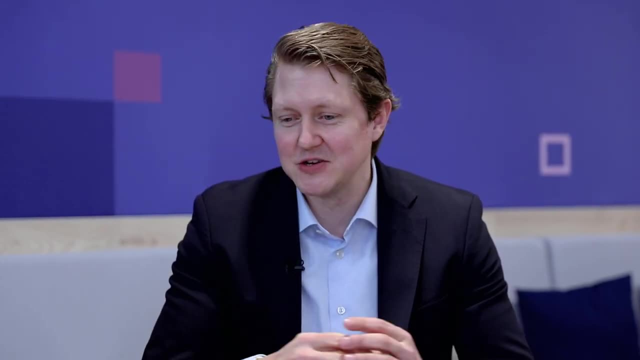 work with partners for the hardware piece And it probably means that the innovation cyclism is accelerating a lot. Yes, it's moved to software. Yes, So the telecom industry is always very interesting to working. I sometimes refer to it as whitewater rafting. You just have. 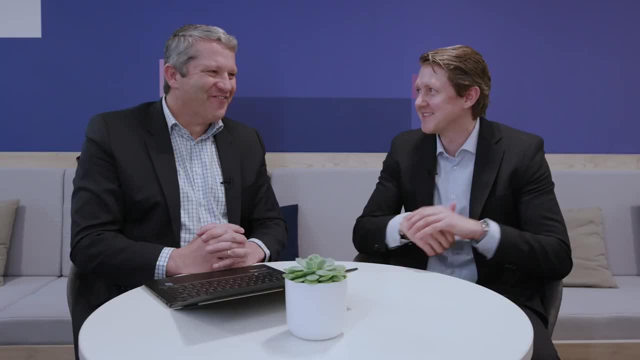 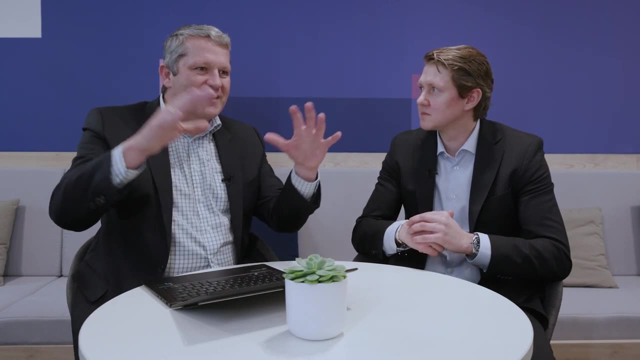 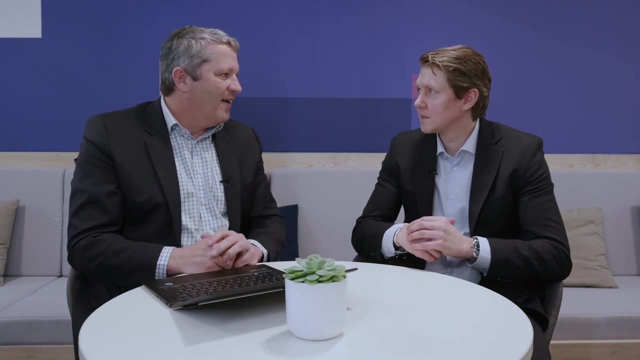 to go And I feel that the water is going faster and faster for every year we're here. Yeah, I feel the same way. So maybe if you come to the Mobile World Congress right now, you would listen in to conversations. You would hear people talk about 5G, 6G, VRAN, ORAN Can. 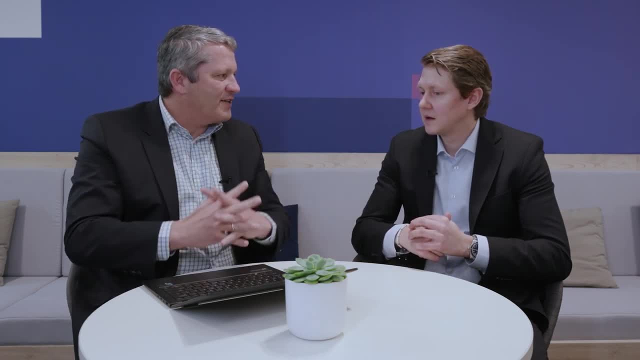 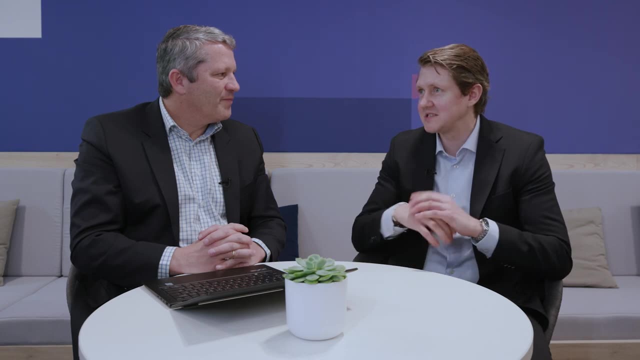 you put that into perspective? What does that mean And where is Ericsson going? Absolutely So. I think 5G and all of the stuff you're saying- 5G, 6G, VRAN- is really the center of the show this year And a lot of the discussions we are having with partners. 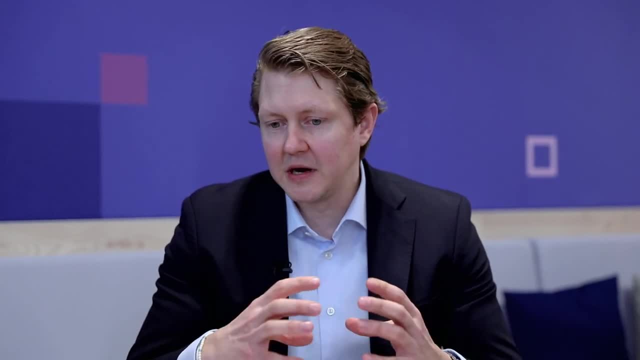 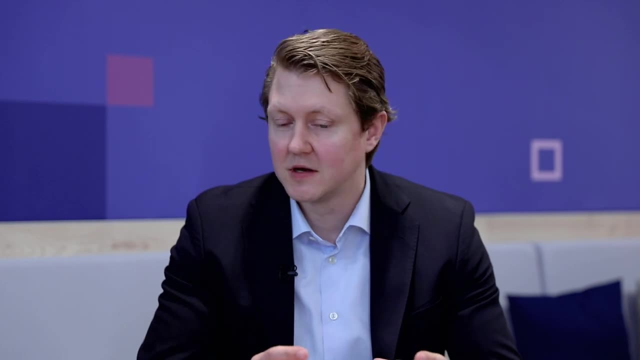 and customers are really centric around this topic, And many of our customers have spent quite a lot of effort of building out their 5G network, their Cloudify, their core network, And everyone is now looking at what's the next architecture that we're going to build for the future. 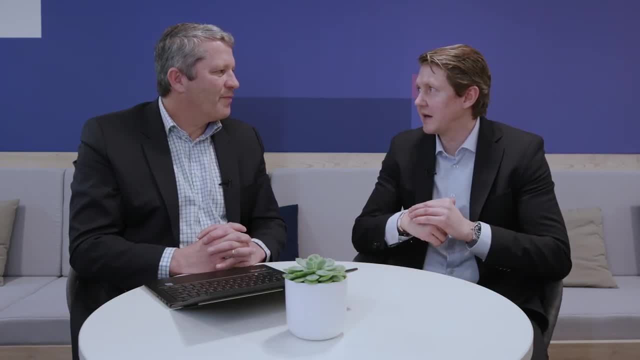 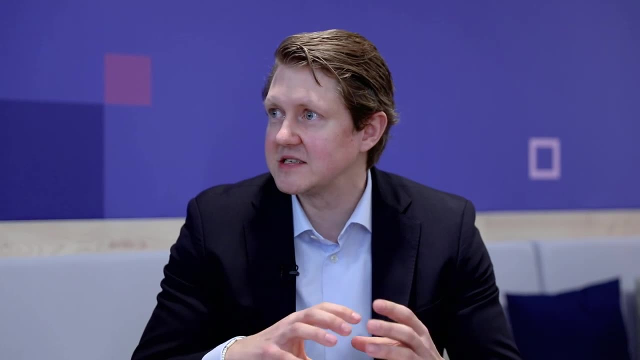 Yes, And this is where Cloud RAN and Open RAN really come into play. We had to spend quite some time now in the industry to try to define what this will be, And I think now is where we're starting to see that this is actually realizing and where we can actually start to see that. 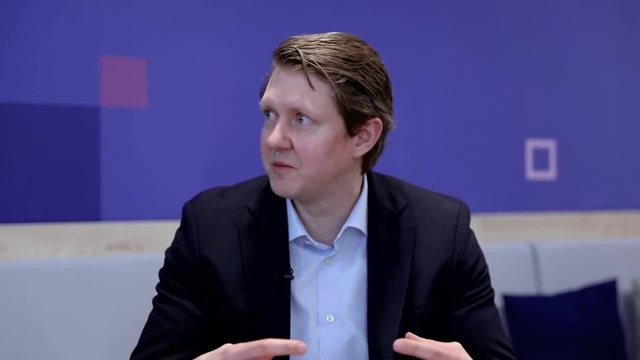 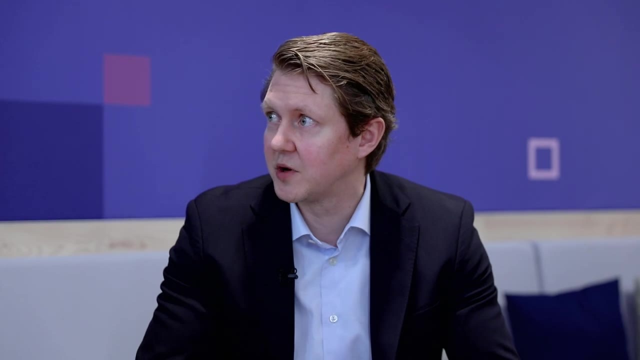 we're picking up the pace and actually look at: okay, so what does the solutions mean for me? What does it mean for my ability to build 5G network? But also what does this mean for my evolution of the network as I go forward into 6G. And that's why the collaboration between our 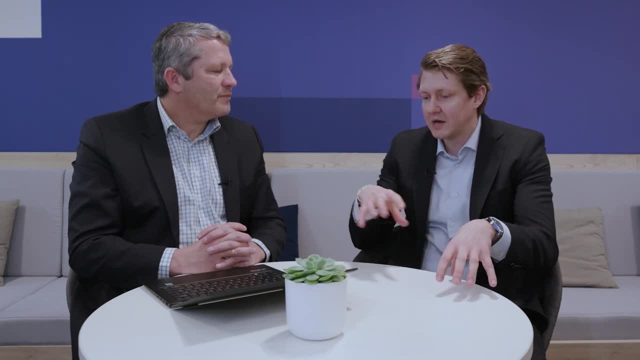 portfolio that we have already out in the market. what we call, then, the purpose-based portfolio and the Cloud RAN portfolio is to seamlessly inter-work, So we can easily introduce this into the 5G network that is there today. Yes, 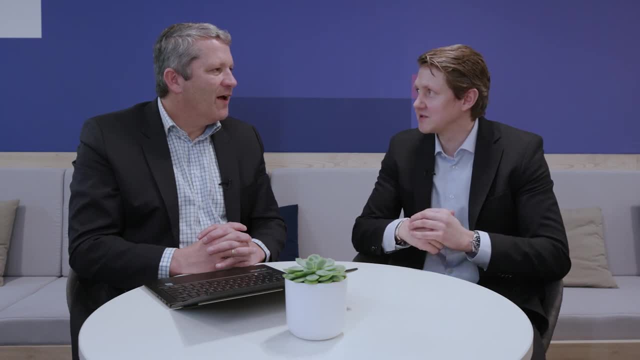 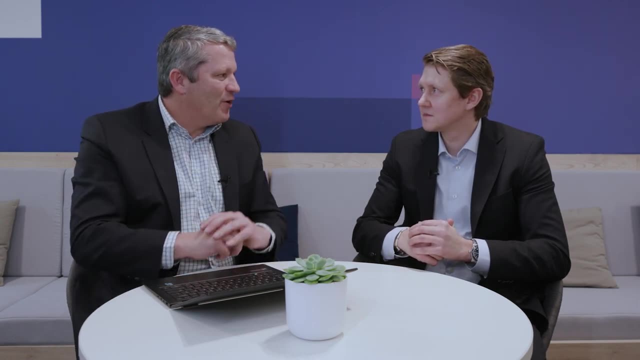 And that is where this whole thing is coming together for the future network tonight. Yes, For me. what is so interesting? I spend in my life a bit of time on digital manufacturing and building private networks, And the dream was to have 5G. Okay, Now we have 5G and we see all of. 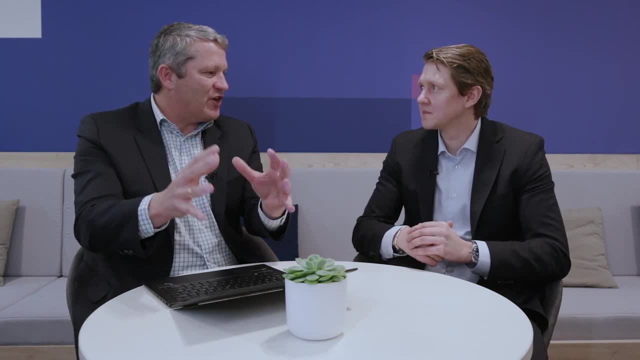 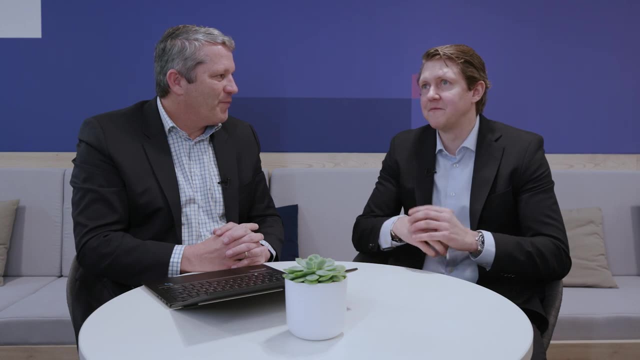 these use cases on the edge and all the AI that can be done on the edge actually become reality And it's super cool for you probably to see that as well happening. It is, It is And it's a major focus on our customer base as well. We have been talking. 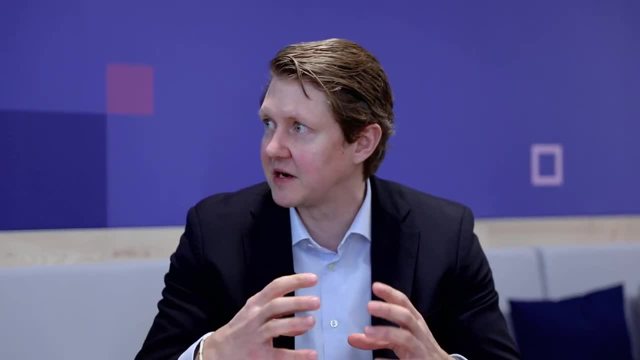 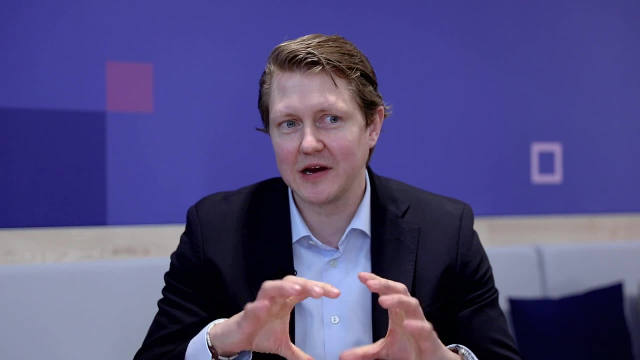 about this 5G use cases and the affinity to monetize the investment that is then going out in the network And I think that, being lifted, what we now are doing with moving out compute without closing to that creates a foundation to realize the potential that is infired. 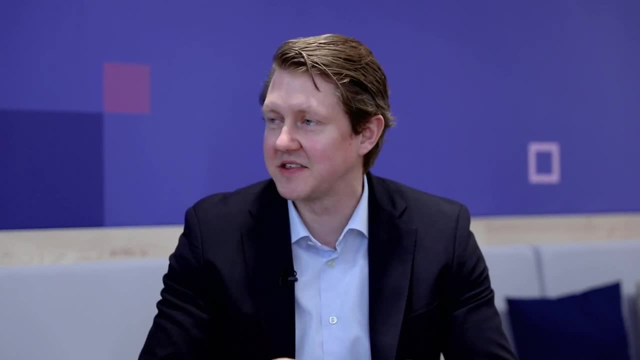 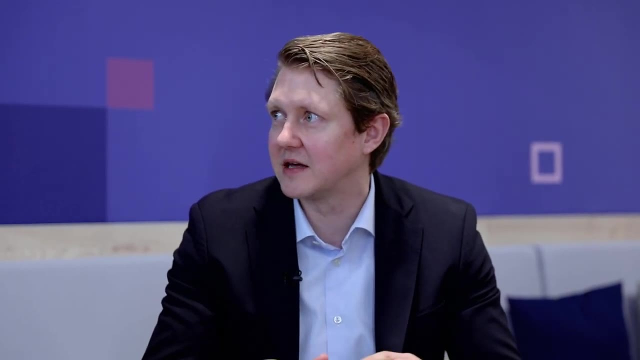 We have to say that we haven't fully done that as an industry yet, and I think that's what we're going to do now. next is to advance the platform as a BIF. let's leverage that for innovation and like, continue on building on that platform. And there AI comes as a very important piece, both when it comes to our own life. 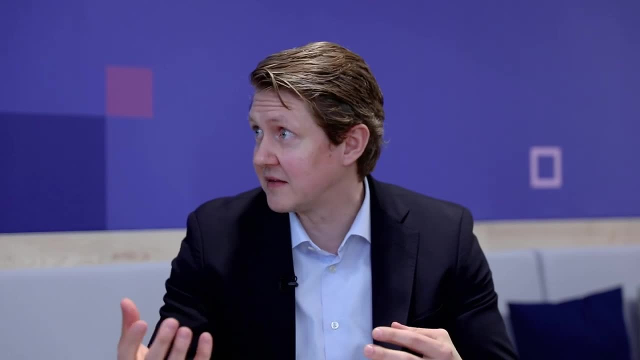 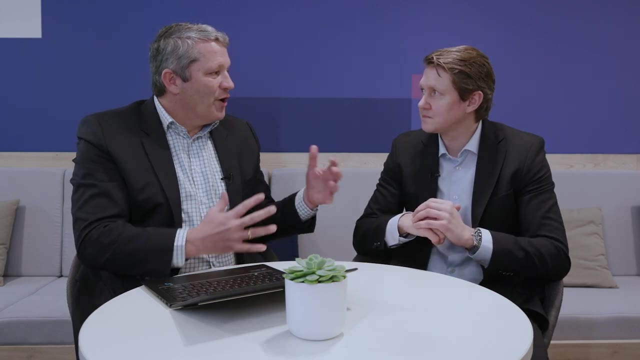 important piece, both when it comes to our old portfolio, but also into the enterprise space, where you can actually then realize some day I components out of this solution. yeah so, Arten, you work with your team very closely with Intel. how would you describe this? how is this going? 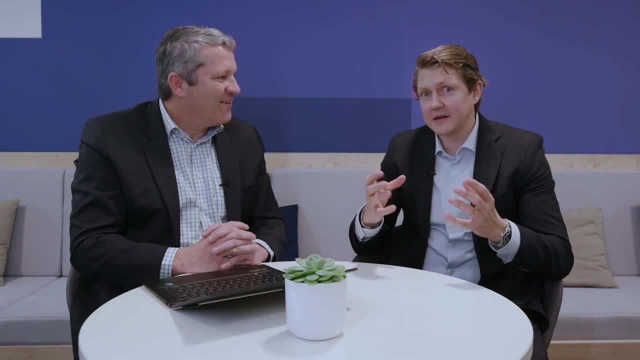 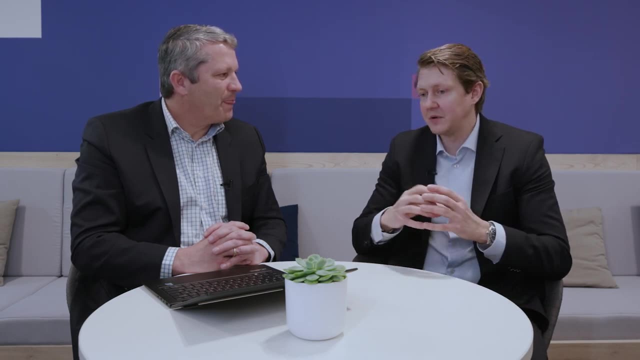 where can we do better? it's uh. first of all, I would like to thank everyone at Intel for this collaboration. I think this kind of very good collaboration. we're working closely together, so it's been really a way for us to realize this architecture. we could have done it without you. 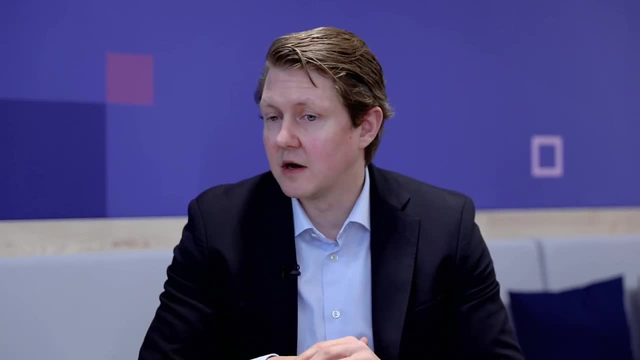 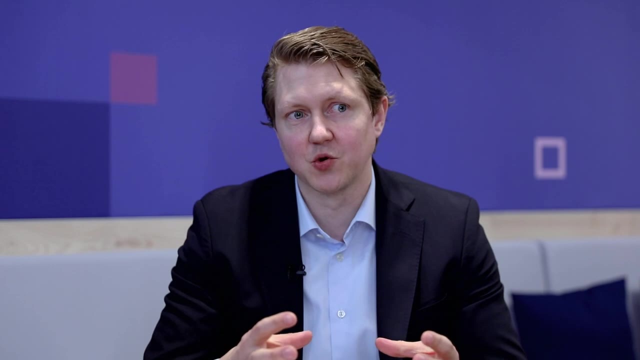 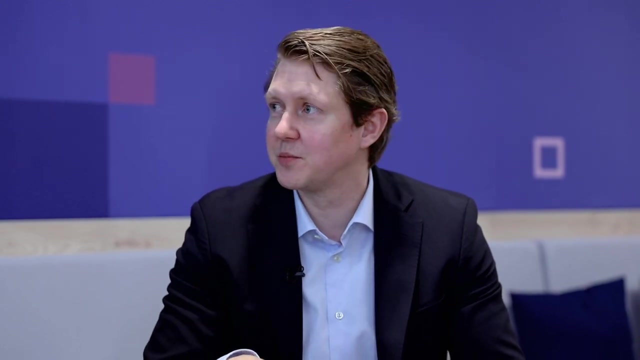 then I have to say that this is also a competitive market. yes, so we see a lot of different players out there today, so competition is going to be free us, and together we're gonna have to make sure that we continue this collaboration. we can't be complacent just because we have a solution now. we have a very good start performance, but the 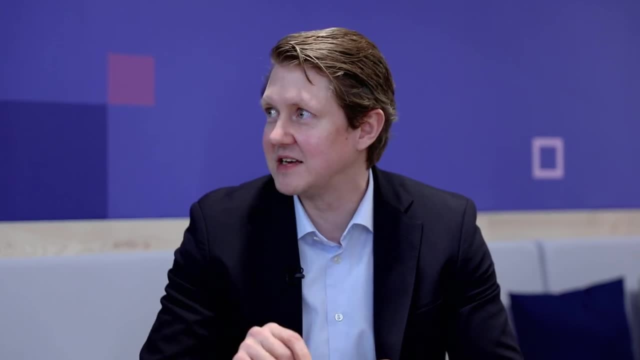 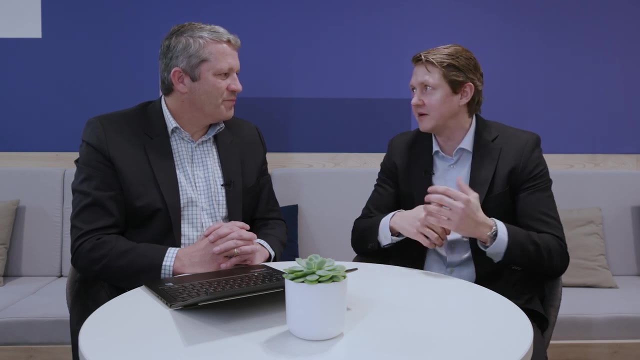 evolution of this is going to be the thing that is going to determine if we succeed or if you fade, and I think the new processor that you're releasing in Barcelona, the fourth generation cyber processor, could only be with a v-run boost. it's a fantastic platform. now we can show that. 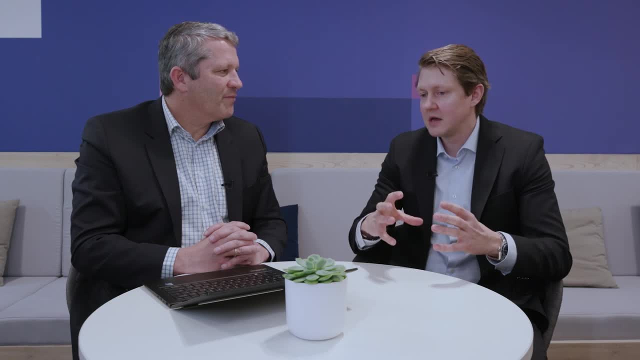 they can actually realize a wrong workflow. that is complicated, but we need to look at the evolution as well. so I really encourage all the innovation and infant to continue to innovate, continue to be able to compete against the competition, but it's going to come into this space and making sure that 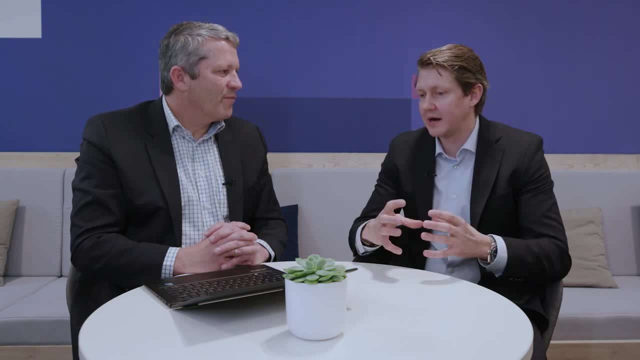 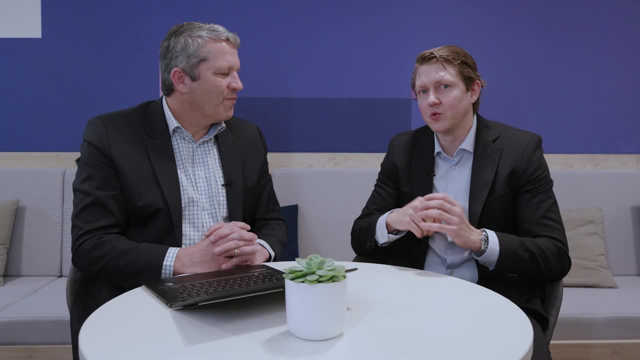 the multi-generational approach that we have in the collaboration can realize not only the only the current solution, but also the future solution, to say competitive feedback. well, that's my number one loss. my number two loss is that we look maybe beyond the power performance aspect of 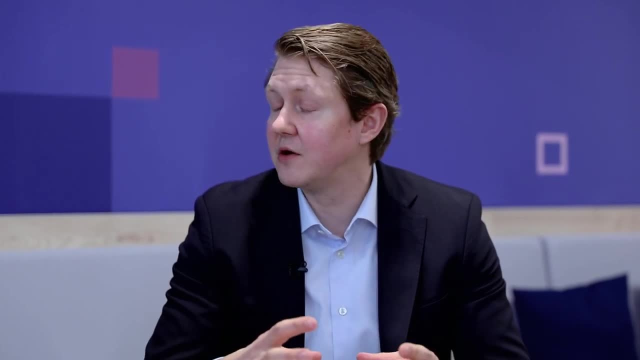 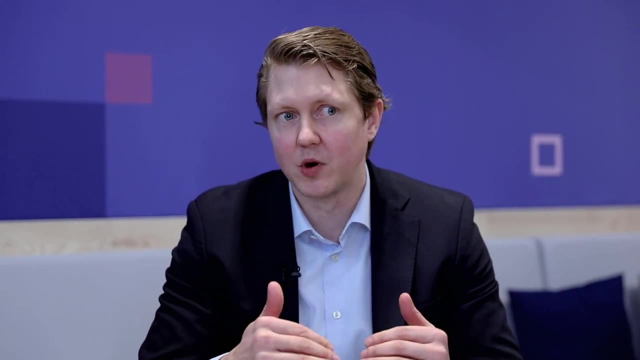 this- because a lot of this will also come into play- of how do we together realize AI solutions and how do we work in the sustainability angle and all of these different dimensions. that is important for our customers in their selection of architecture and that's where we need to. 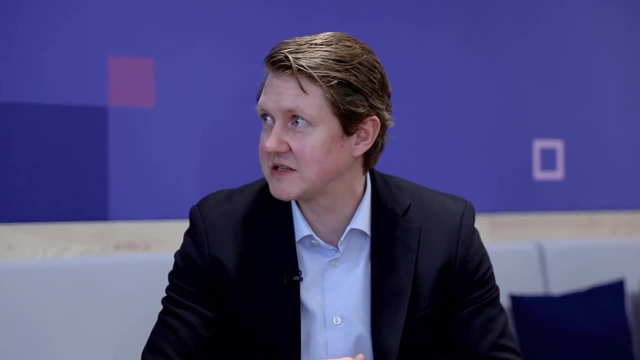 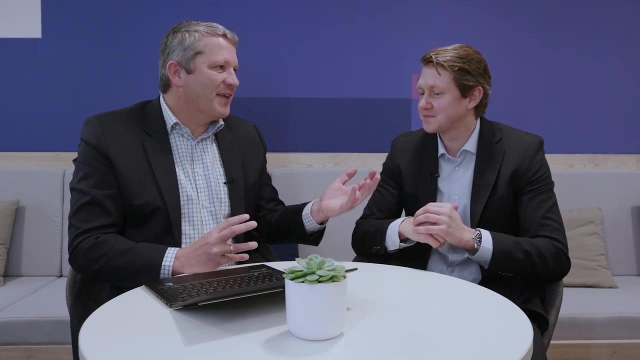 collaborate together. we need to never stare. it's on you, well, tech cup, that we have established board innovations like this. and make sure that we get tangible deliverables out of it- yes, but I think tangible. and also making sure that we bring real value to our customers, yes, and that we bring 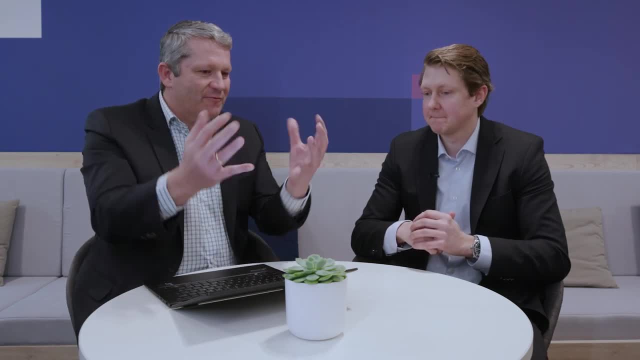 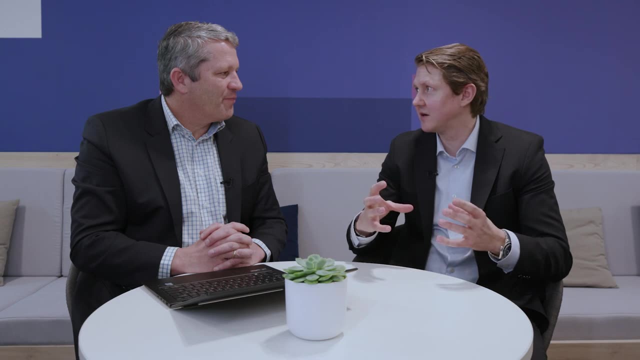 value that we can then continue to build on and make these relationships very, very sticky. yes, I fully agree. I think we have a. we have a good starting point. we have seen our CEOs being on stage to talk about how we're now going to stand this for industry scale and make sure that this 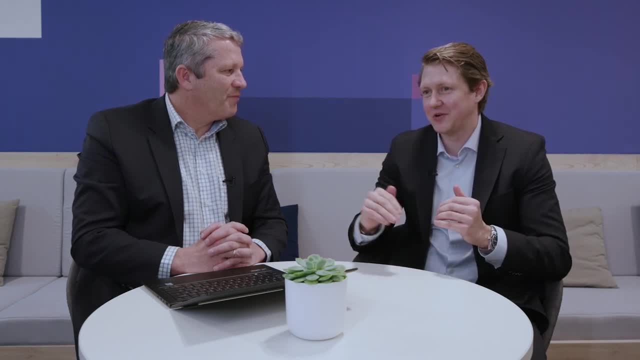 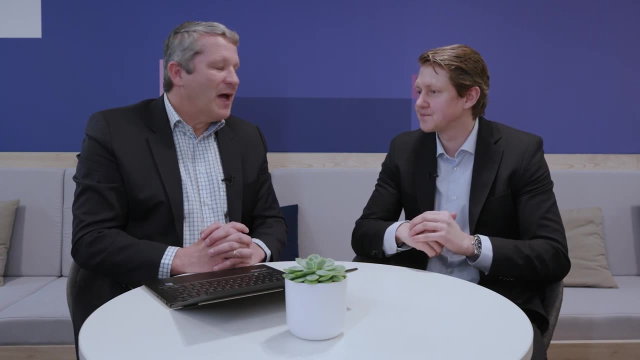 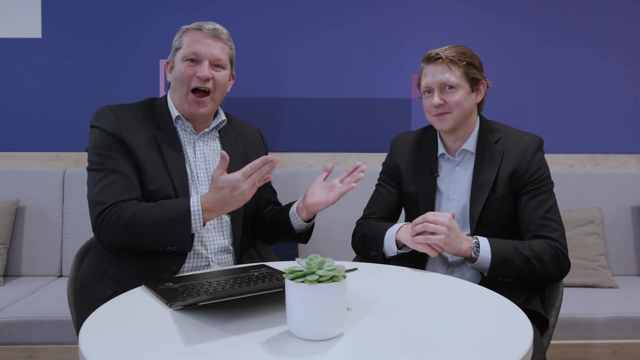 become a solution, but we also have to build on next generations as we scale and as we get this customer discussions going. it's not the end of it, it's the start. that's a start. I agree with you, Martin. thanks so much. I really appreciate you joining me and I hope to all of you that you learned something listening, uh, to our customer. 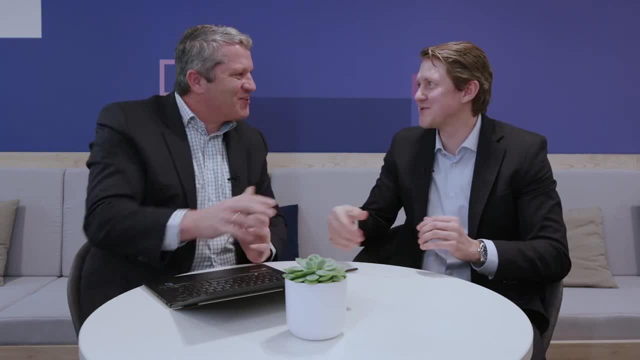 Martin from Ericsson. thank you so much. thank you for having me. thanks for coming. it's great, thank you.